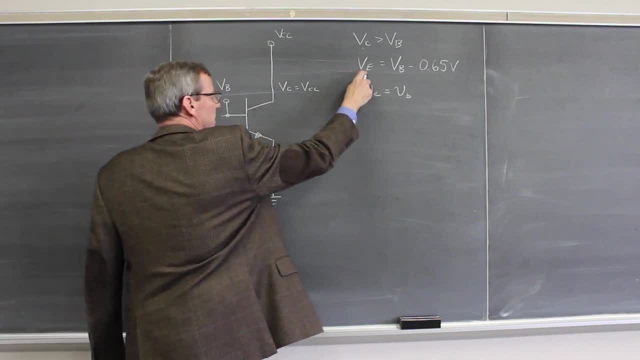 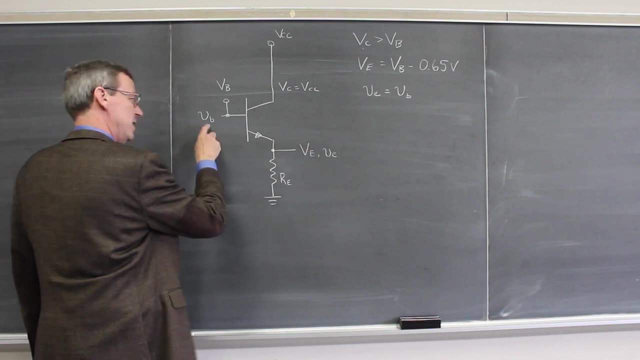 the emitter voltage and you get a diode drop across here. So the emitter voltage DC level is the base minus one diode drop, 0.65 volts. And if we put an AC signal VB in here we get an AC signal VE. The AC signal VE that comes out of here is simply a copy of that. 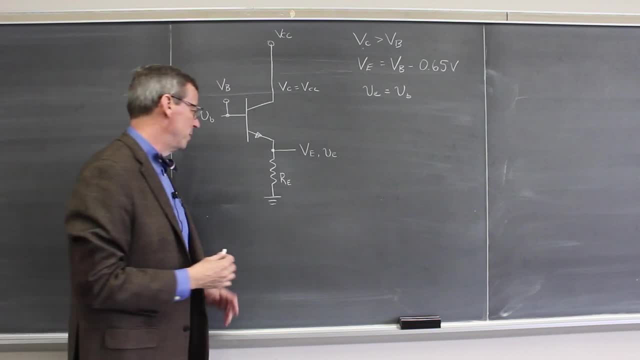 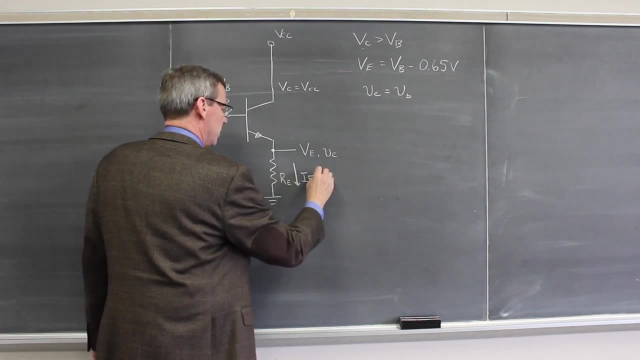 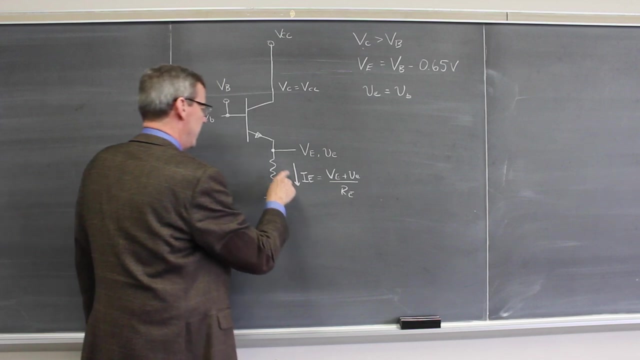 so we get a copy of that there. And the last thing to remember is that the current flowing through this emitter resistor here is VE plus VE over that resistor And that is approximately the current flowing into the collector. Remember, the base current is about one percent of that. 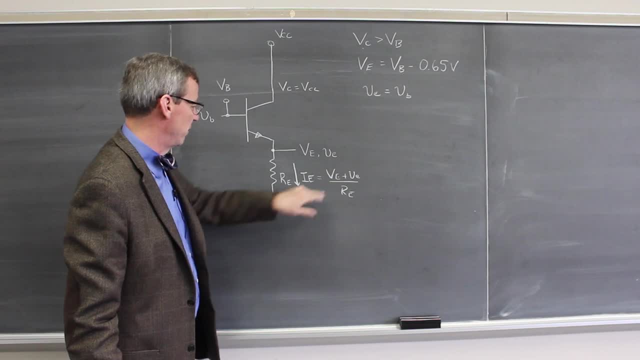 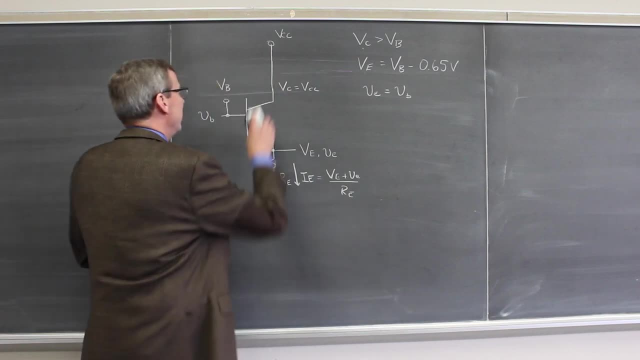 so most of the current is here. So the emitter current and the collector current are both given approximately by that. Okay, What we're going to do now is we're going to vary this a little bit. We're going to add a resistor between the power supply and the collector, We'll call it RC And we're 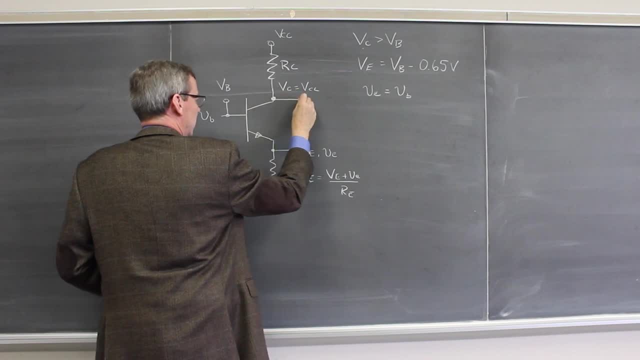 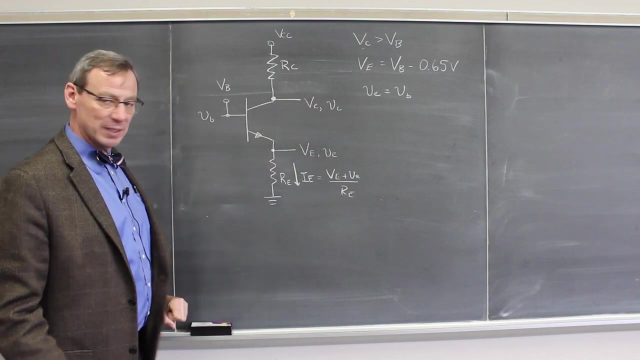 going to take the output at the collector, So there will be a V collector and presumably an AC signal And presumably the collector voltage. The collector voltage is no longer going to be a copy of VCC, So we won't be doing anything with the emitter anymore. We'll be looking at the collector And we can simply write. 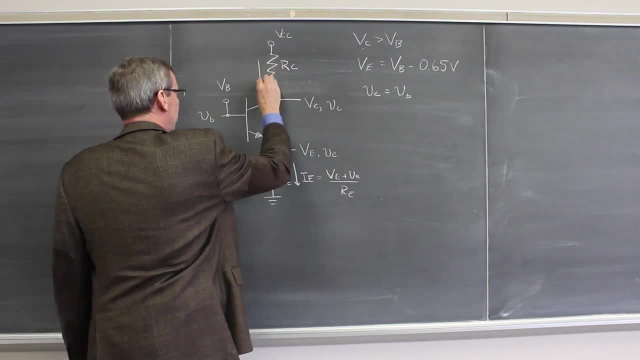 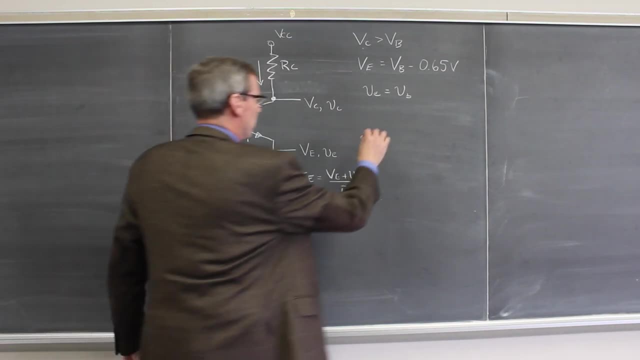 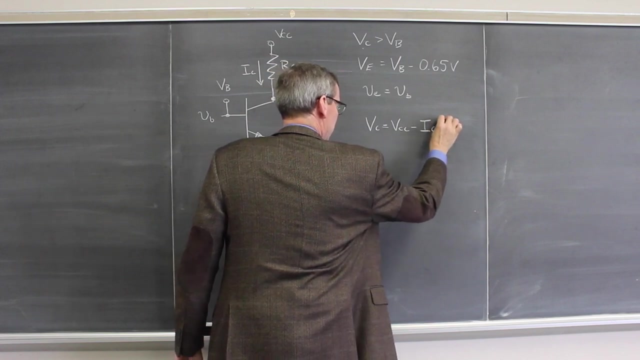 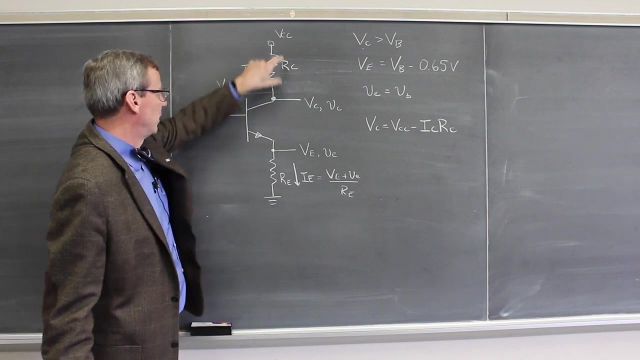 down here the collector voltage is whatever current is flowing through that resistor. times that resistor is the voltage drop. So the DC collector current has to be VCC minus ICVCC RC. Okay, So that's the DC level there. So this is lower than the collector voltage. 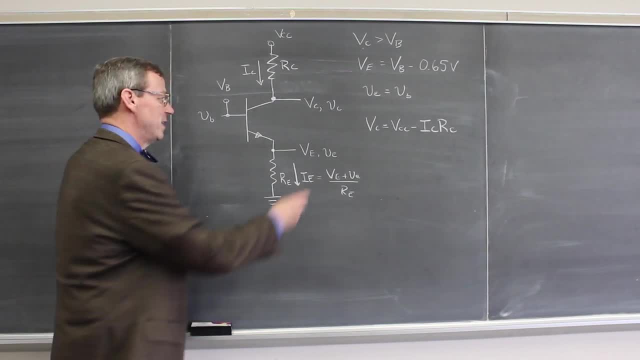 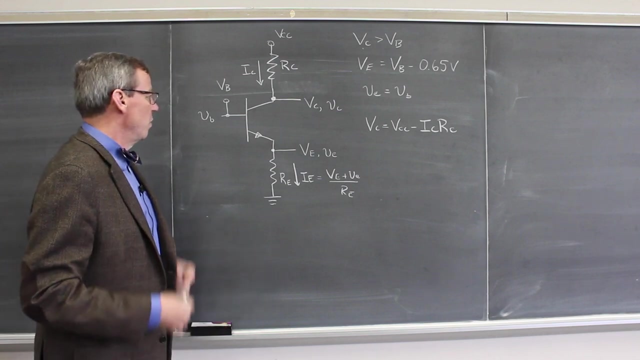 by whatever the current flowing through there is, And to keep the transistor biased, this collector voltage still has to be bigger than the base voltage. that would bias. So that's nice, though That biases this, And we still have the same relation. Whenever we set the base voltage, the emitter voltage is 0.65 volts. below that We can obviously 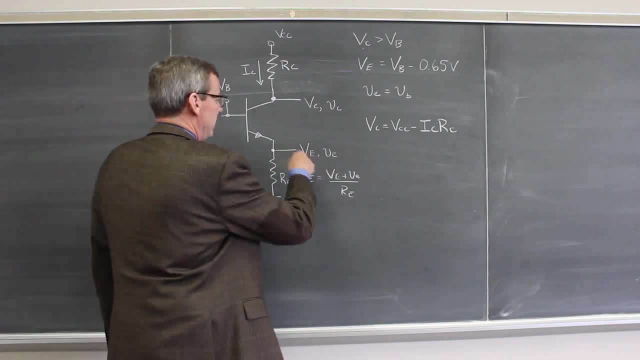 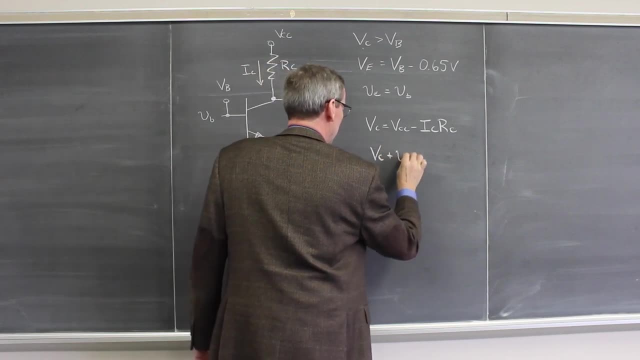 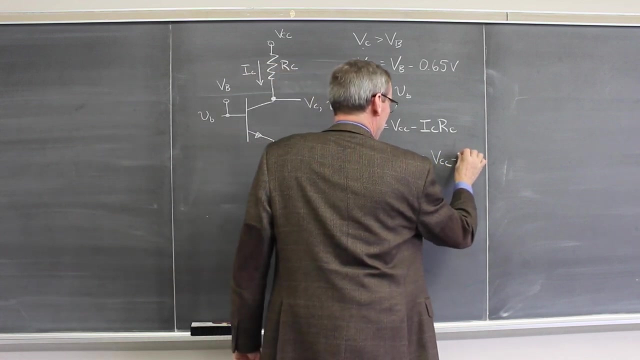 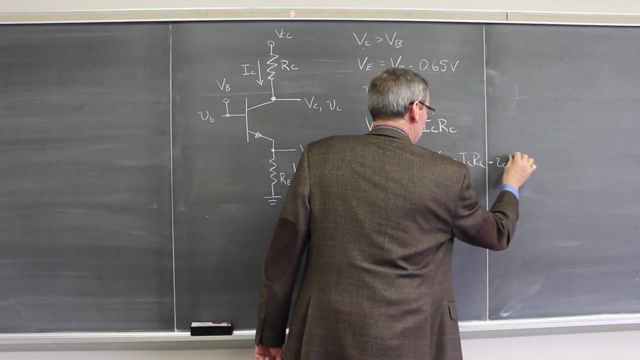 extend that if we put an AC signal in here, There's going to be an AC signal here, presumably there's an AC signal here. so the VC plus the AC signal is going to still be that DC level minus the DC current, and now we're going to also get the AC current. 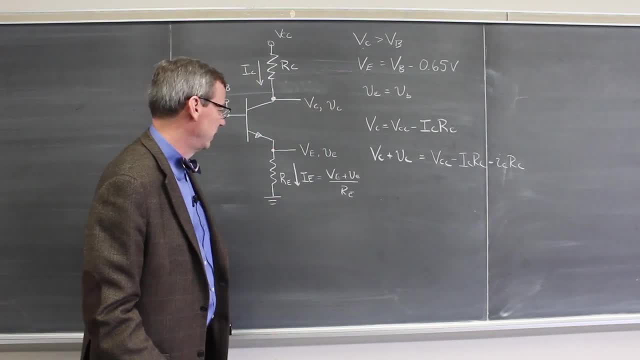 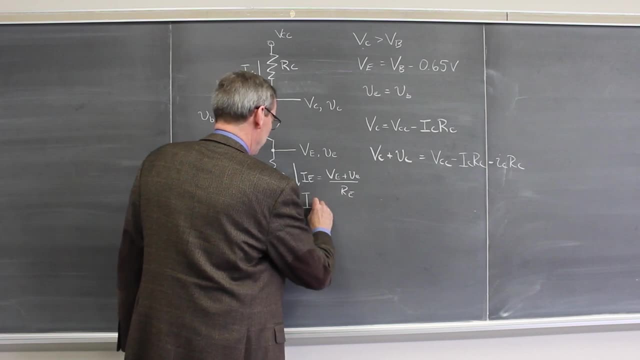 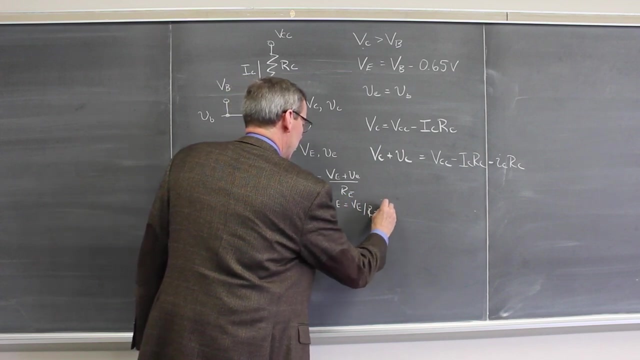 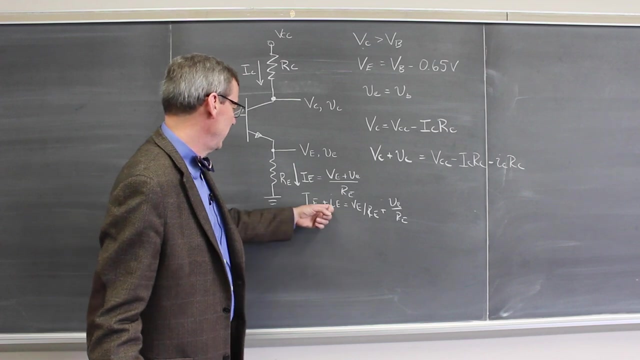 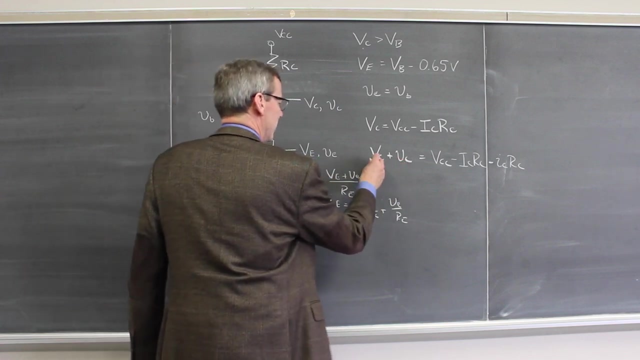 subtracting from that. okay, so we get something exactly like that now that current here. I just should have written this actually as IE plus IE is VE over RE plus little v. so there's the DC- current VE over RE, there's the AC- current little VE over RE, and I can now do a couple of things. I can separate this into the DC. 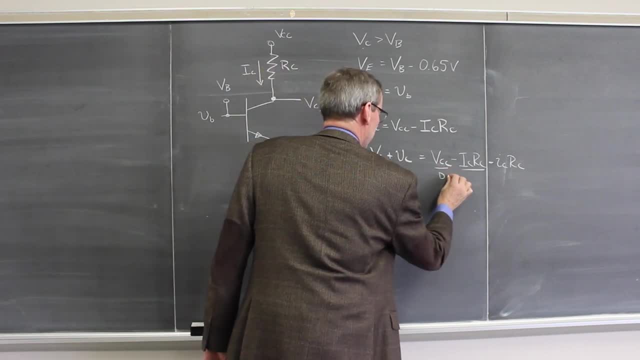 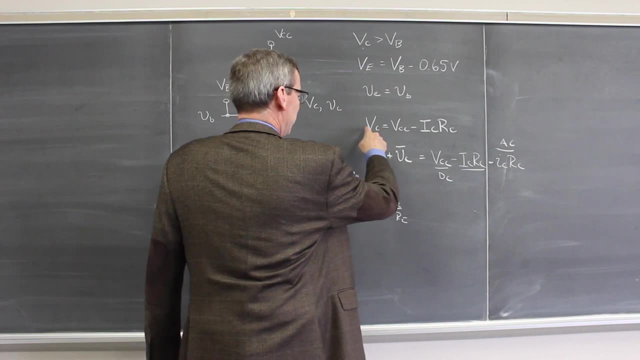 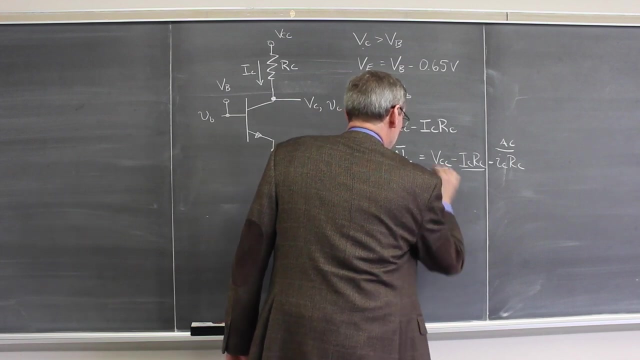 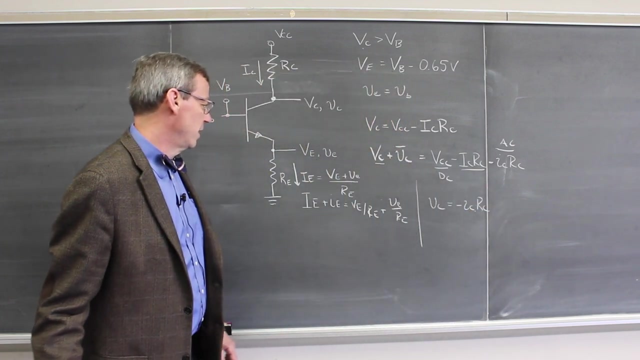 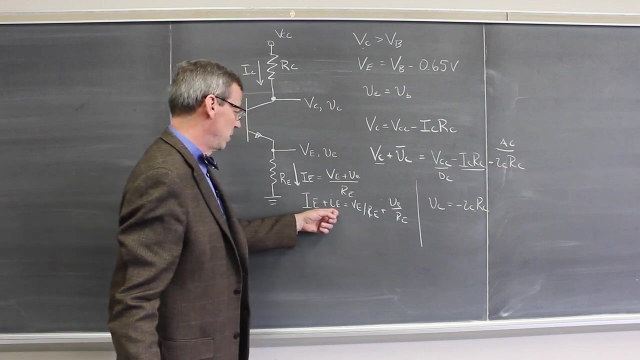 parts. so that that and that are all DC, DC and that and that are AC. okay, so I have. the DC gives me exactly the same relationship I had before, and the AC now gives me VC is minus IC RC. okay, that's nice there. now the collector current is pretty much equal to the emitter current. 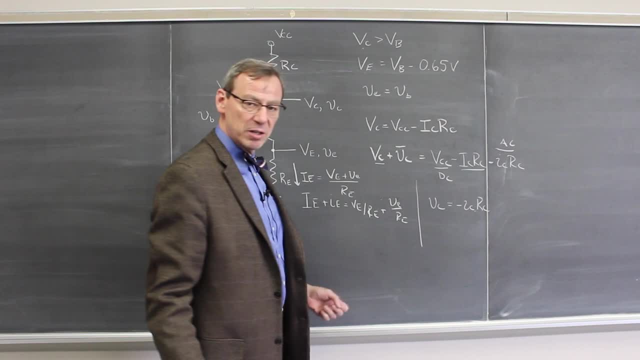 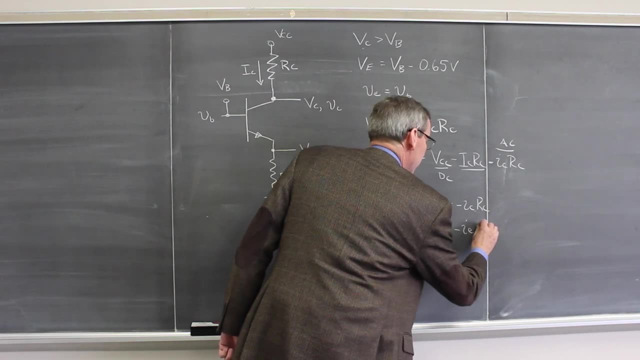 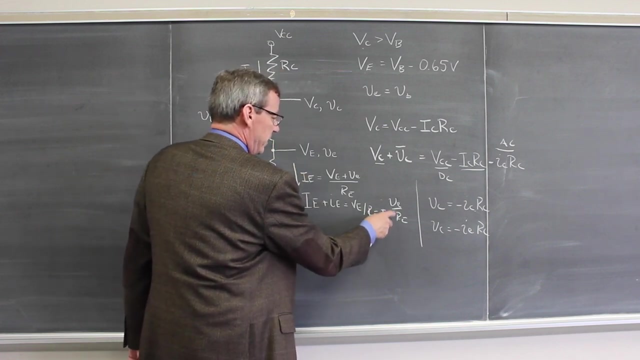 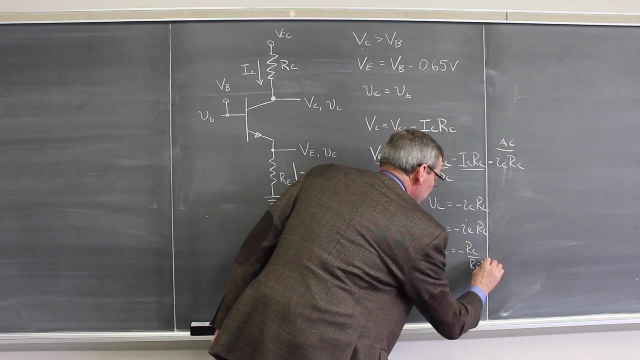 so I could replace the collector current with the collector current and I could actually write this: VC is minus IE, RC, and then I can put in what that is in terms of the AC voltages VC, it's going to be minus RC over RE times, VE. okay, so 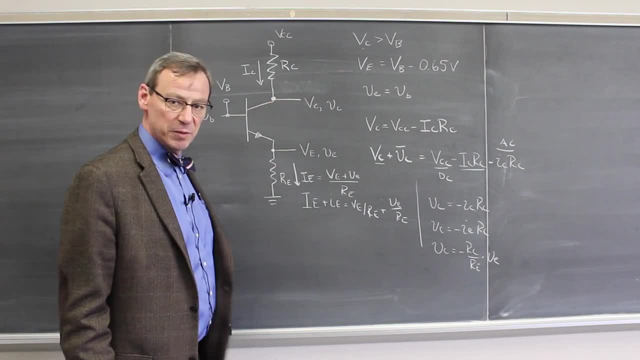 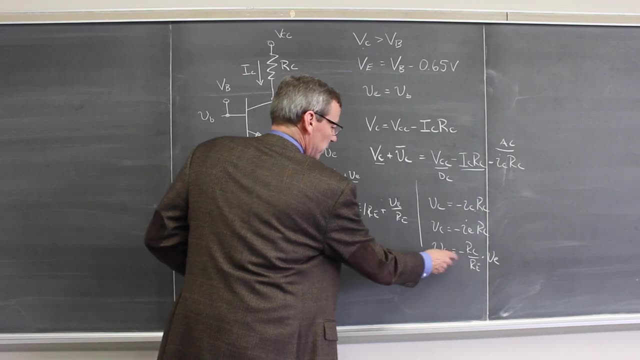 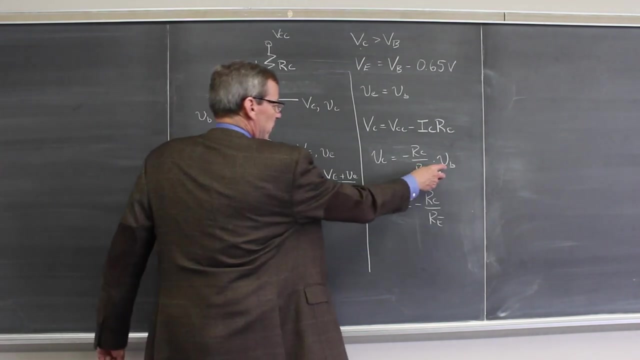 that now gives me a relationship between the collector voltage and the emitter voltage, but the emitter voltage is still just a copy of the base voltage, so what we're going to get is that the collector voltage is the ratio of these resistors times the base voltage. so if we replace the emitter voltage with the 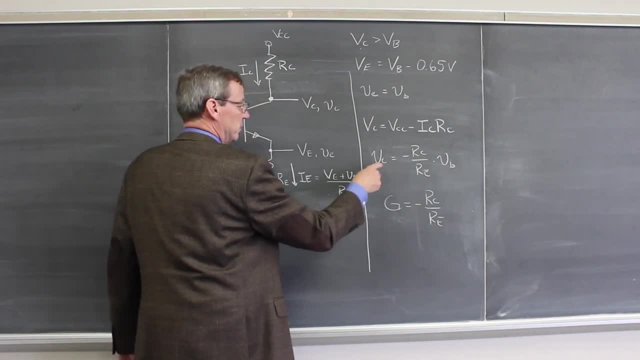 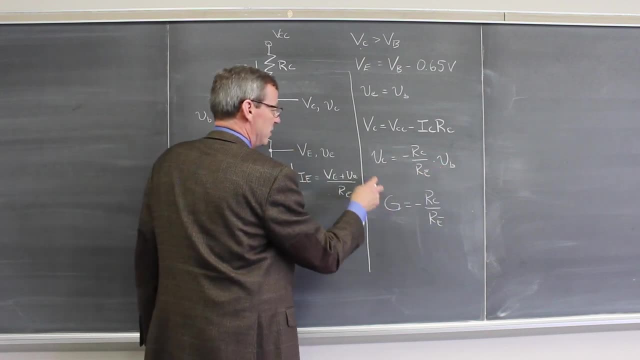 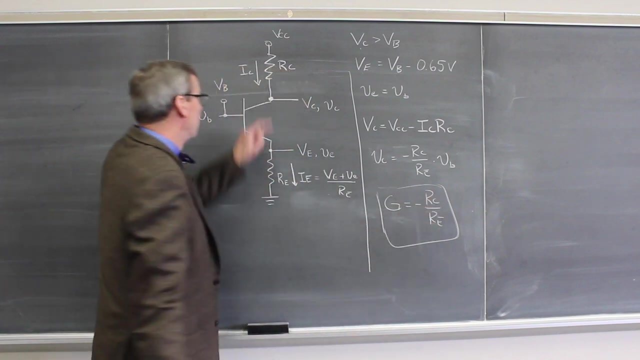 base voltage, which is just a copy. then we get this relationship here that the collector voltage AC part is the ratio of RC to RE times the input voltage and that just says the gain is the ratio of the output to the input or minus RC over RE. so if we choose RC to be bigger than RE, the output AC signal will be bigger than. 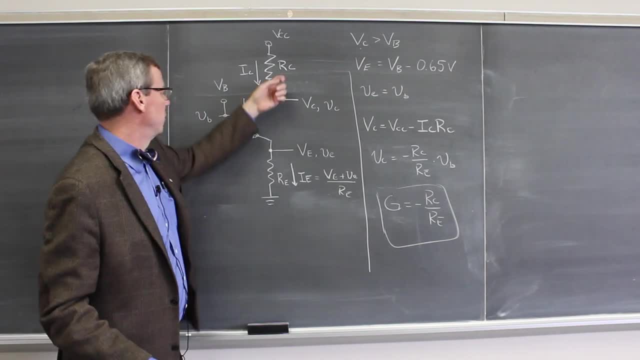 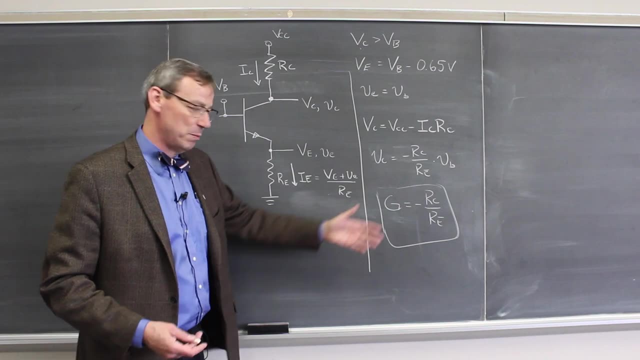 the input AC, we get an amplification. so if we chose this 10 times bigger than this, we'd have an amplification of 10. the minus sign just tells us that the trig function on the output is inverted from the trig function on the input. we